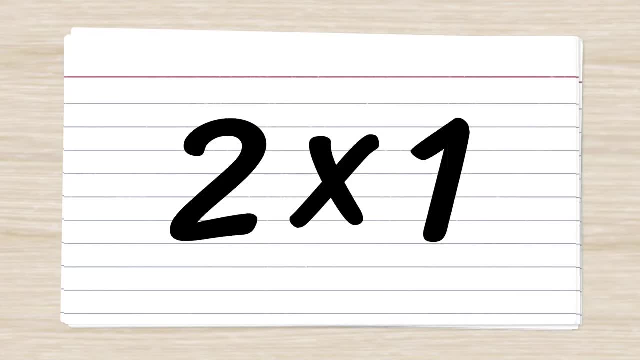 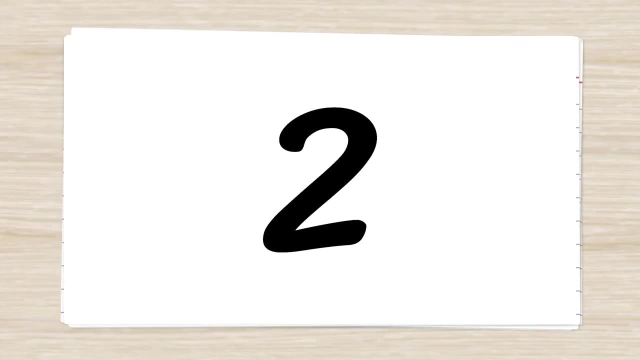 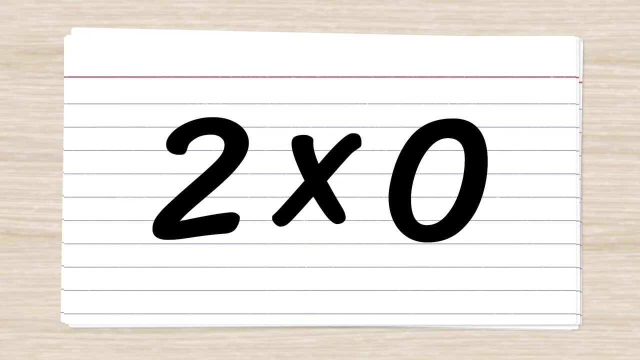 12, 2 times 1, 2, 2 times 5, 10, 2 times 10, 20, 20, 2 times 0, 0, 2 times 2, 4, 2 times 4,. 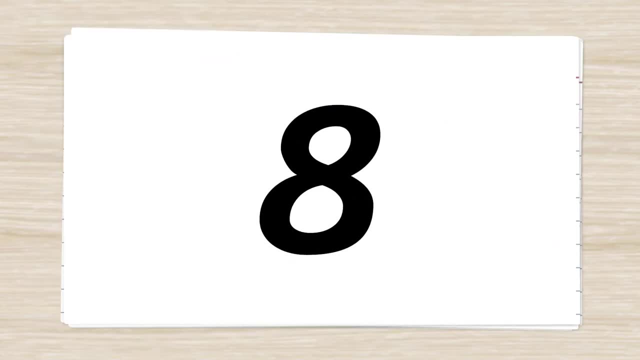 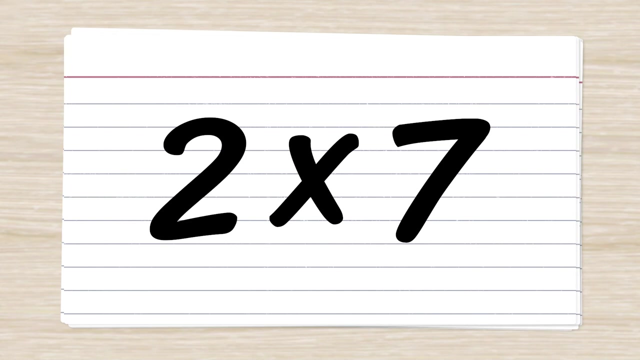 8, 2 times 3,, 6, 2 times 7,, 14, 2 times 8,, 16, 2 times 4,, 8, 2 times 3,, 6, 2 times 7,. 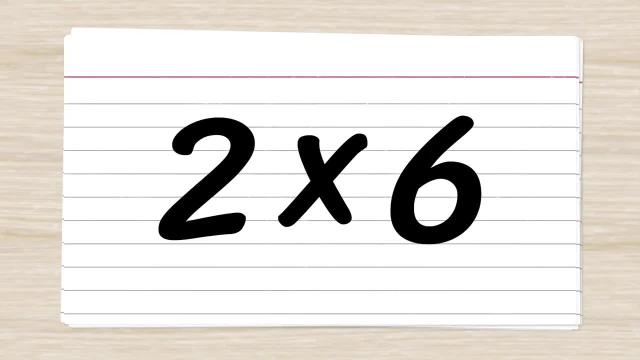 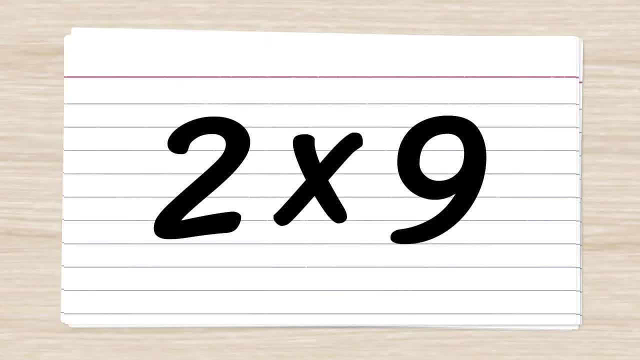 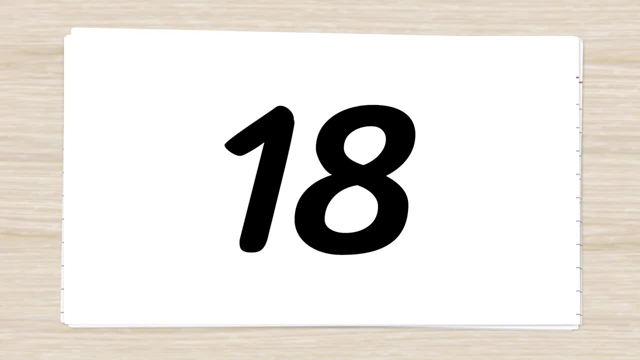 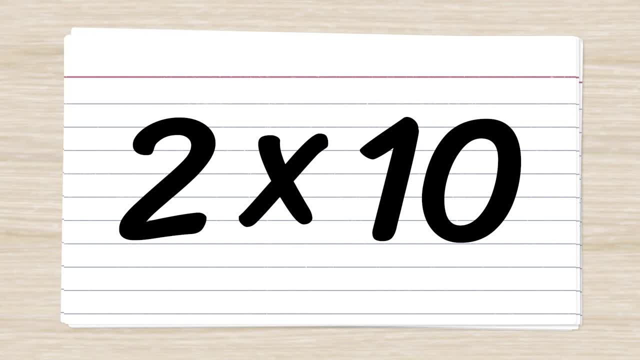 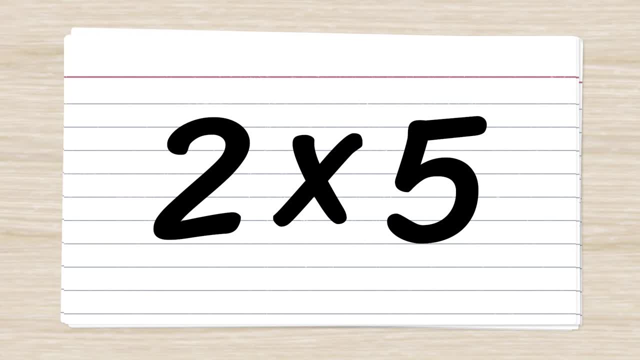 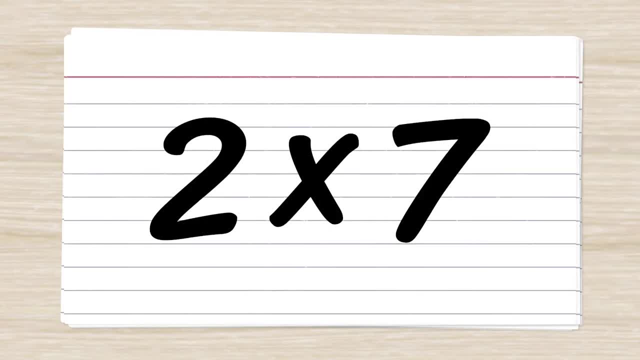 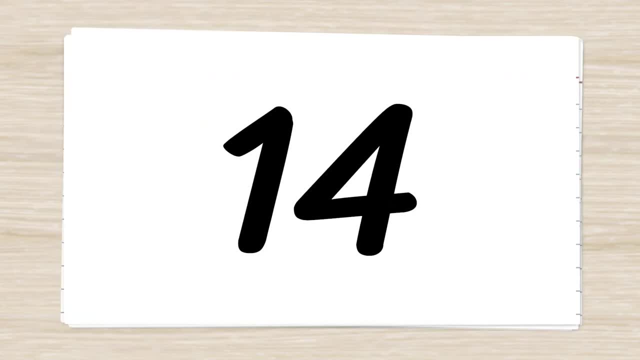 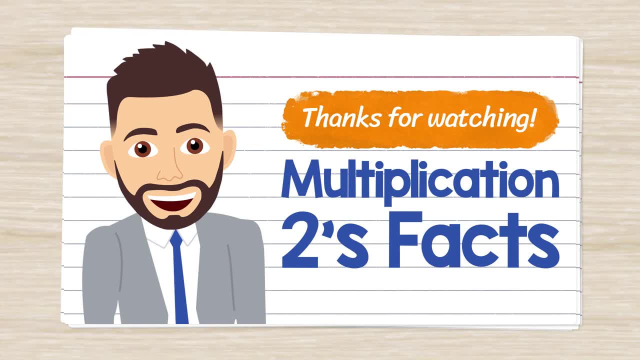